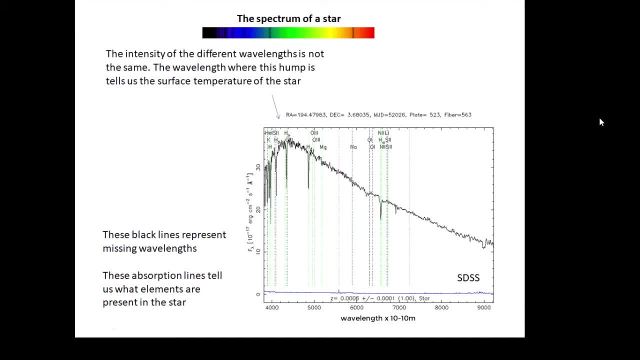 ROYGBIV. but you get a hump. Basically, you don't get the same amount of each wavelength. There's a particular wavelength where there's a maximum intensity and this is very interesting. The position of this hump tells us the temperature of the star, Basically, the the bigger the wavelength. 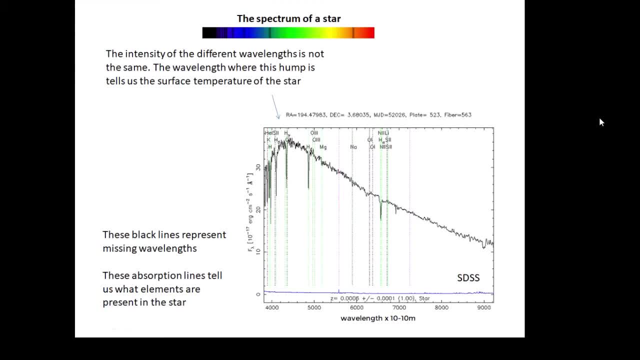 where the hump is, then the cooler the star, The smaller the wavelength. where the hump is, then the hotter the star. So we get this hump okay. Another very interesting and very useful thing is that there are black lines on the spectrum. There are wavelengths which are missing. 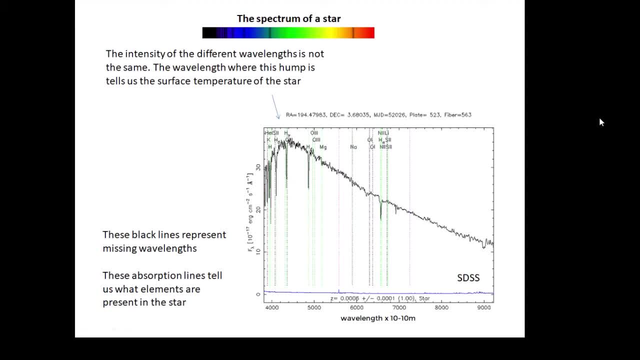 and these are very important because they tell us what elements there are present in the star. We can actually figure out what the star is made from by looking at the, the position of these black lines. We call it an absorption spectrum In 1814 Joseph. 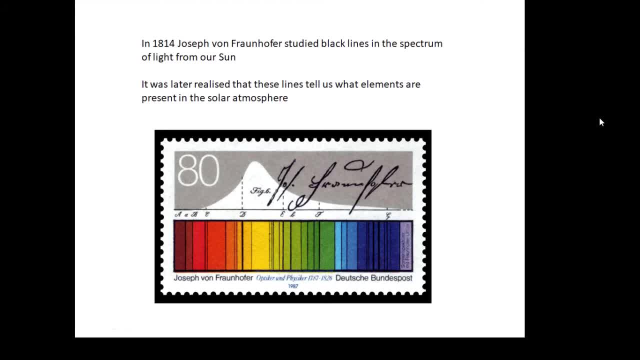 von Fraunhofer found these black lines in the spectrum of light from our sun. I don't think he was the first person to see them, but he studied them and he made lots of measurements of them, and later on it was realized that these black lines in the spectrum of our sun tells us 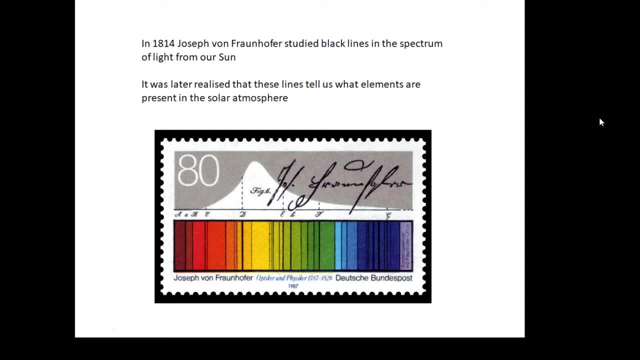 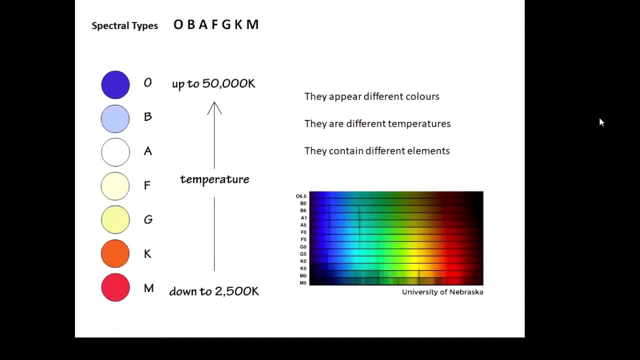 what elements there are in the atmosphere of the sun, which was how helium was discovered. So what spectral types are there? What are the different types of star? O B A, F, G, K, M. The easiest way to remember it, very traditional way: O B A. 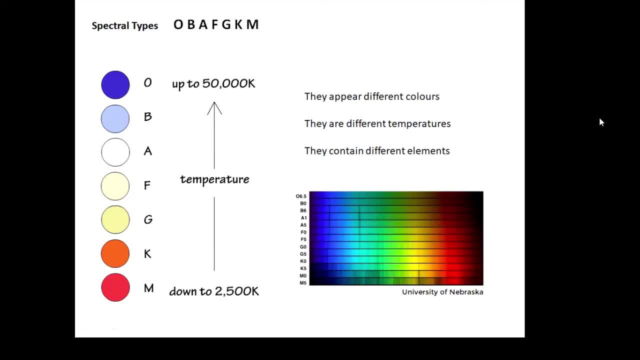 fine girl, kiss me. Okay. and these are the different types of star, These different types of stars. you should learn the colors. the very hot ones, up to 50,000 Kelvin, are blue. The the much, much cooler ones are red. The ones in the middle are kind of white and yellow.